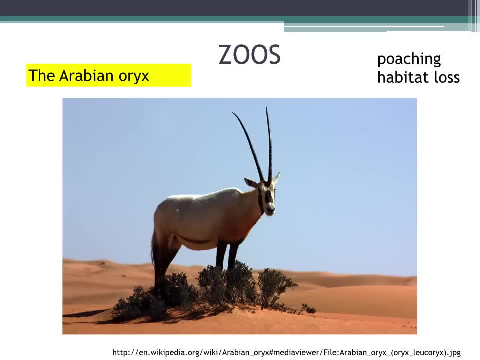 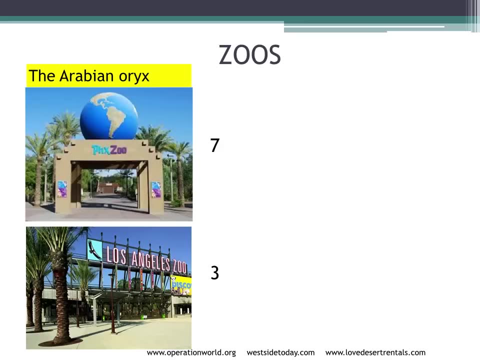 However, using zoos, breeding programs were set up and these animals were reintroduced into the wild. It was found that the Phoenix Zoo had seven left and the Los Angeles Zoo had three. They initiated a breeding program and reintroduction was done through the Zoological Society of San Diego into Oman. 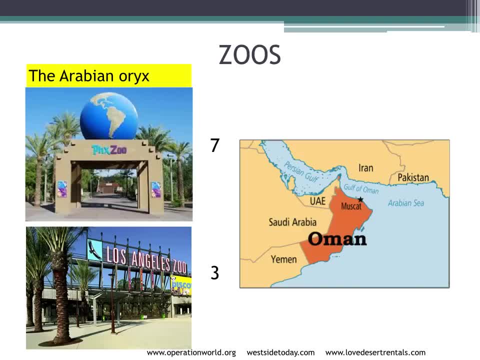 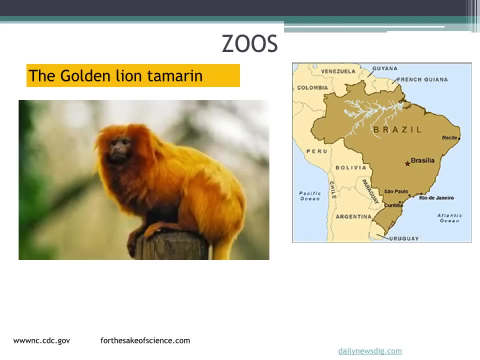 Now there are more than 1,000 Arabian oryxes in the Middle East, with over 4,500 in reserves and zoos globally. The next little creature is the golden lion, tamarin. It's native to Brazil and lives in the coastal forest. 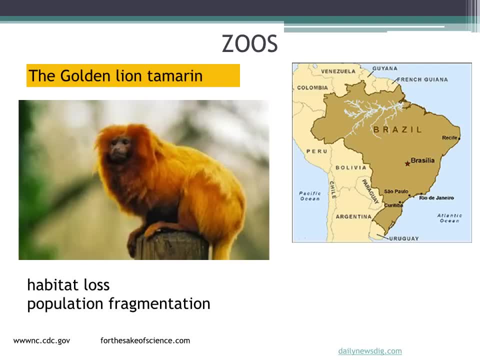 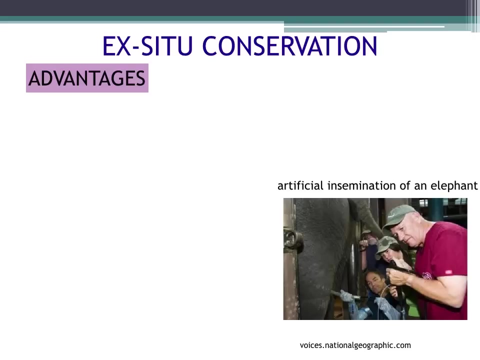 It became endangered because of habitat loss and population fragmentation. In the 1970s there were only 22 in the wild. Through collaborative effort, including breeding programs and habitat restoration, there are more than 1,500.. So we've discussed XC2 colonization. 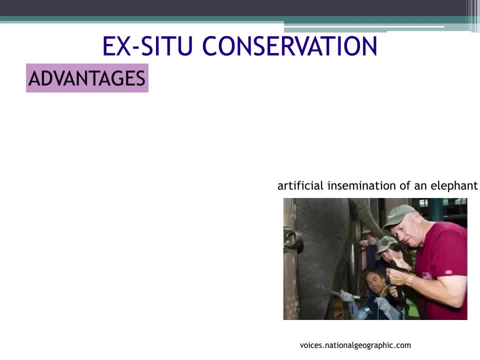 So this is conserving a species outside its natural habitat, for example in a zoo. The advantages of this include using DNA analysis to identify the close species. For example, if you use hybrids in plants, Techniques can be used to place the embryo into the surrogate mother of the same or similar species, enhance ovulation. 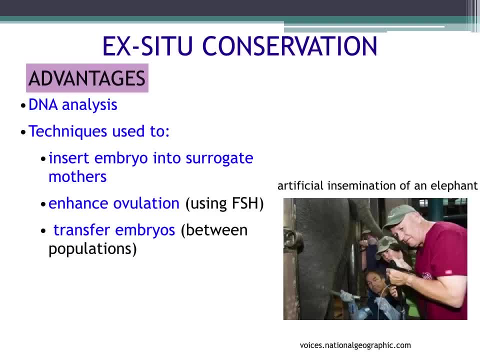 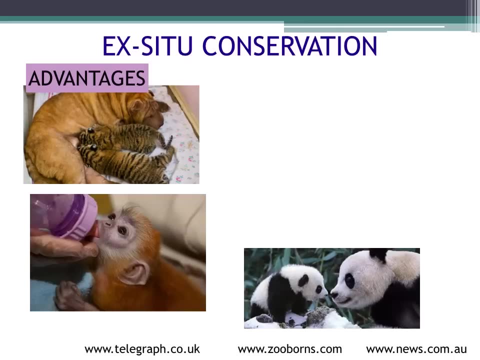 and you can also transfer embryos from one population to another Or use donor sperm from another zoo. This can then be used in artificial insemination or in vitro fertilization. These methods will increase genetic diversity and assist in breeding animals that will not, for various reasons, breed in captivity. 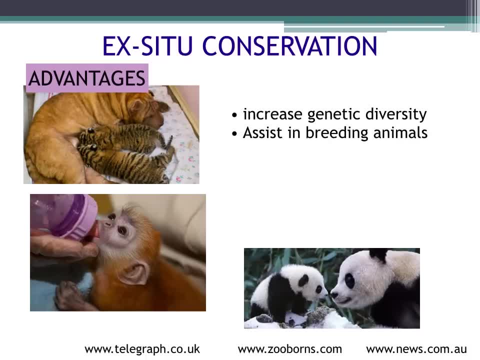 There is the possibility of using somatic cloning and trans-species cloning, which means that the egg and the surrogate mother are from different species, The fetus and the mother can be monitored and provided with the proper care And, finally, genetic records can be kept to prevent inbreeding. 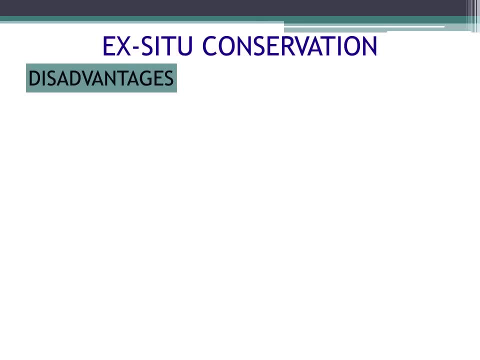 Can you think of what kind of disadvantages there might be with conserving animals outside their natural habitats? Behavioral disorders. Behavioral disorders, Behavioral and genetic problems. Only 26 of the 274 rare species of wild animals are self-sustaining in zoos. 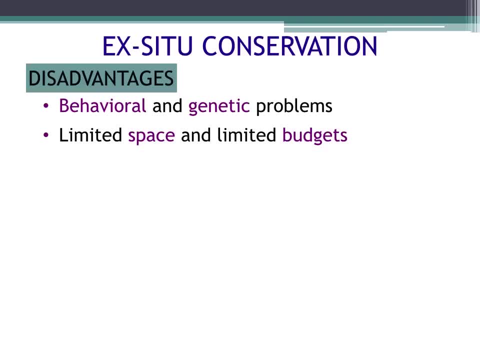 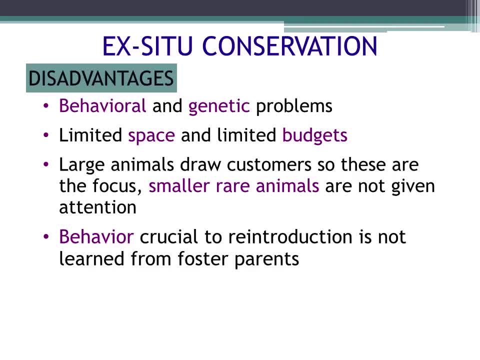 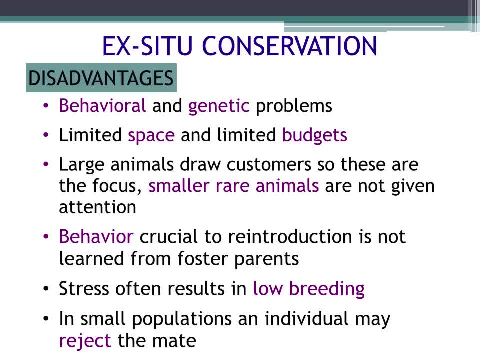 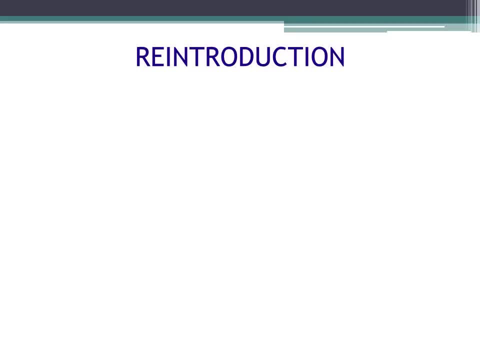 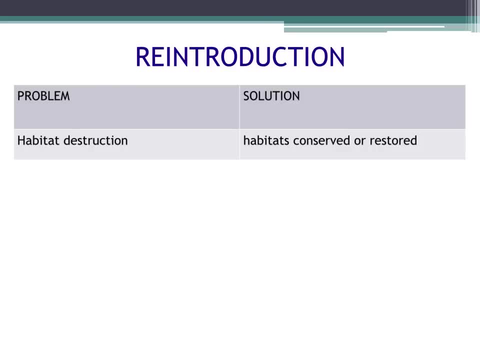 Habitat destruction, So a solution might be to conserve the habitat or restore the habitat. Animals might be unfamiliar with the space or vegetation type, So zoos must be set up with similar habitats. Animals cannot find enough food in the wild, So there should be. 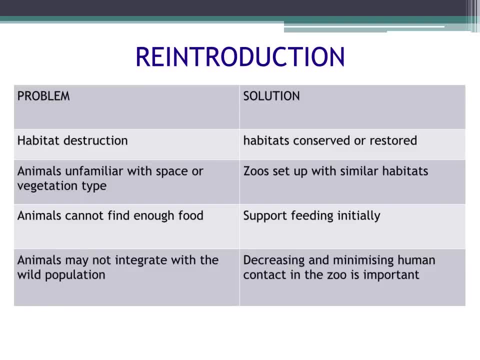 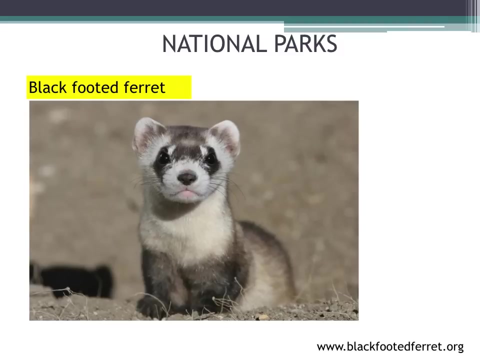 support feeding. initially, Animals may not integrate with the wild population, So it's important to decrease and minimize human contact in the zoo. And finally, animals may be susceptible to diseases, So they should first be acclimatized in cages. The next animal we'll look at is the black footed ferret. This became endangered, But